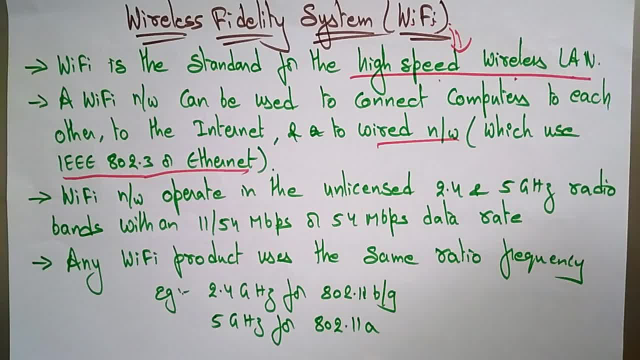 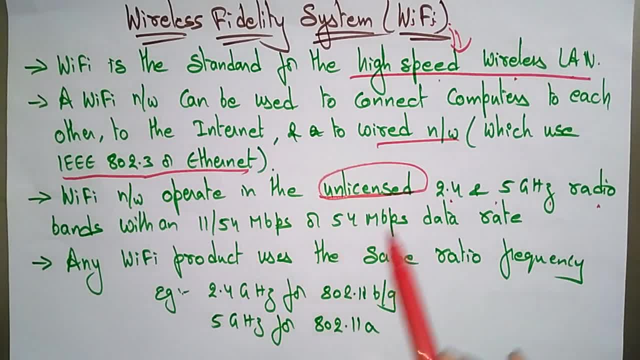 Unlicensed 2.4 and 5 gigahertz radio bands. So why we call it as an unlicensed? because if you want to Use a wireless communication, rooting is sufficient for you, Okay, then you always. devices can be inter-connected by using the. 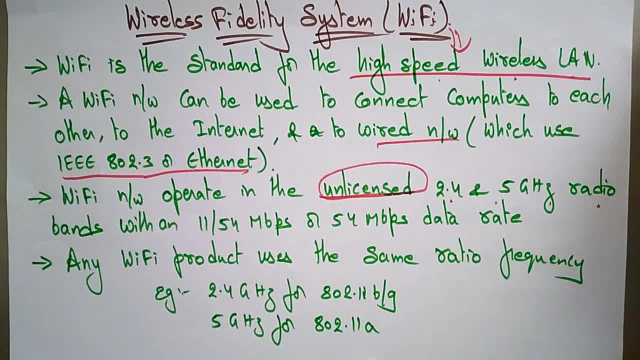 wireless Wi-Fi. So there is no license is required further to connect Hardware to use a Wi-Fi purge optimized. So if you want to use any software you need license. okay, Like Antivirus software or some other software you need to Purchase licenses. but here the wi-fi network operator is in the unlicensed to 2.4 and 5 gigahertz radio bands. 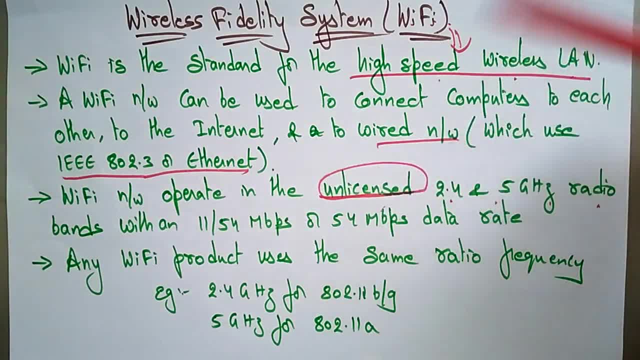 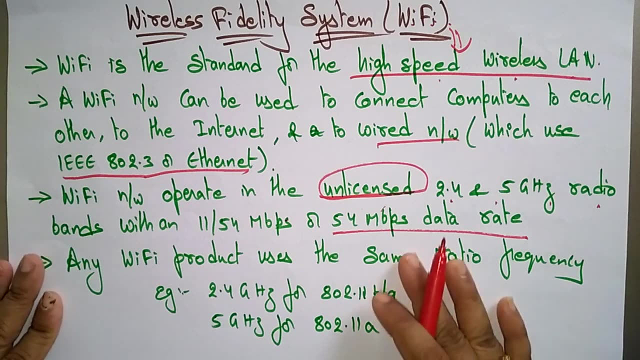 with an 11 by 54 megabits per second, or even the 54 megabits per second data rate will be there for all the wi-fis. so any wi-fi product use the same ratio frequency. the ratio frequency will be same for the wi-fi product. so if you take any wi-fi product that is a 2.4 gigahertz for 802.11. 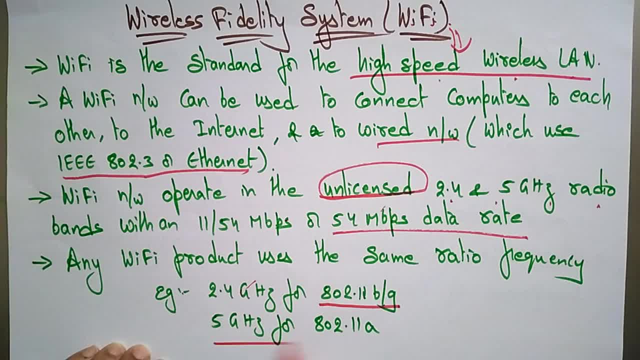 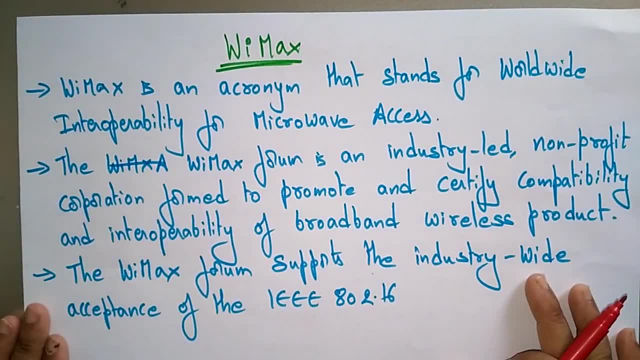 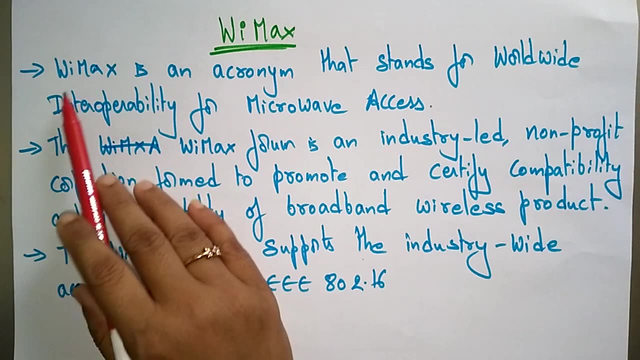 b or g, and 802.11 a, which is a, 5 gigahertz. so this is about the wireless fidelity system. now coming to the next recent advances in wireless network is a wi-max. wireless max max is a microwave. we call it as a. let's see this. the wi-max is an acronym that stands for the. 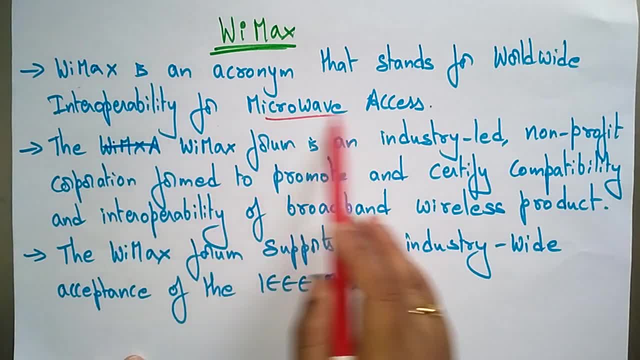 worldwide interoperability for microwave access. the wi-max forum is an industry-led non-profit corporation formed to promote and certify compatibility and interoperability of broadband wireless product. actually, why they introduce the wi-max? the wi-max is just first. uh, it is a non-profit corporation which is formed to promote and certify compatibility and interoperability of.